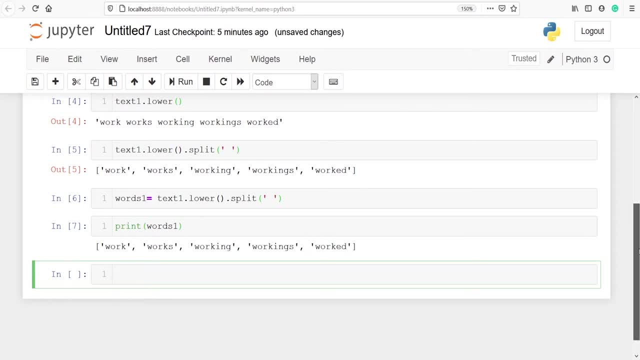 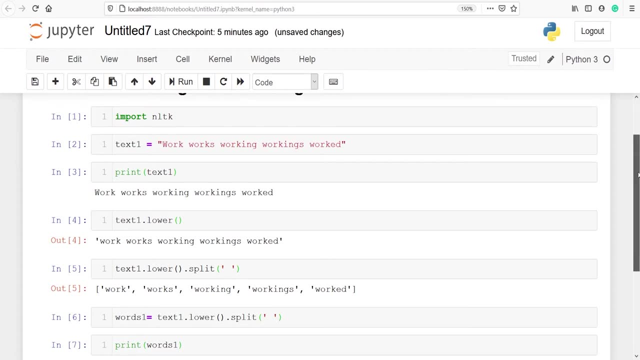 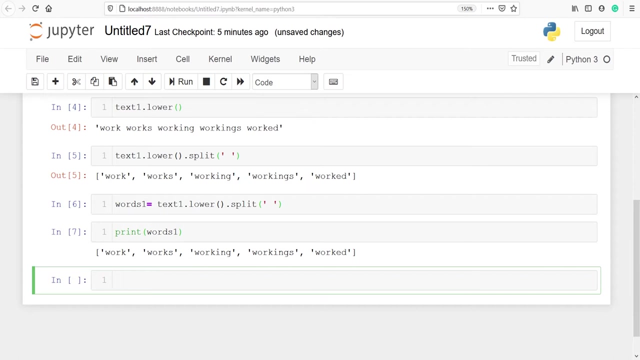 This is normalization, That is, we have normalized all the words. Now no words are like. some words are in capital letter or in small letter, but now all the words are in the small letter. This is the process of normalization. The next is stemming. Stemming is to find the root word or the root form of any given word. 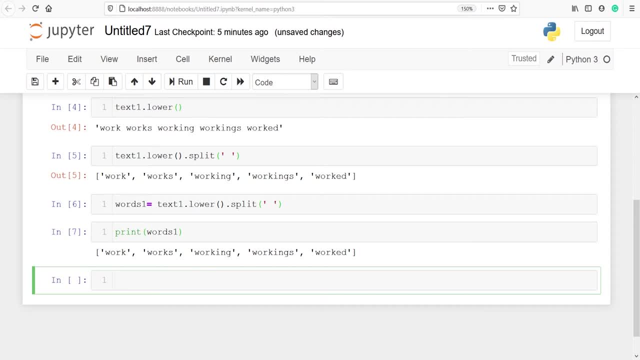 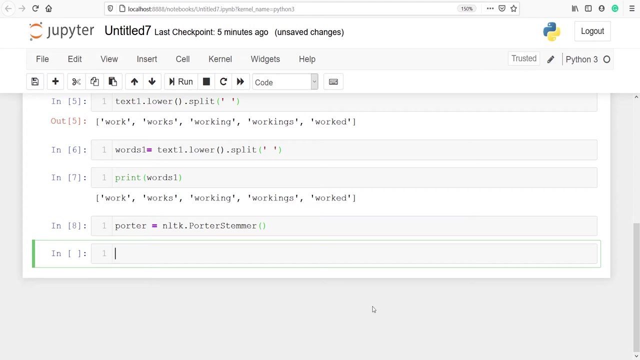 We will import port porter stemmer to do stemming. but there are many other algorithms as well. I'll make one variable porter Now from NLTK. I will call port stemmer. This is a function for stemming. Let's execute our code. So we have saved the. 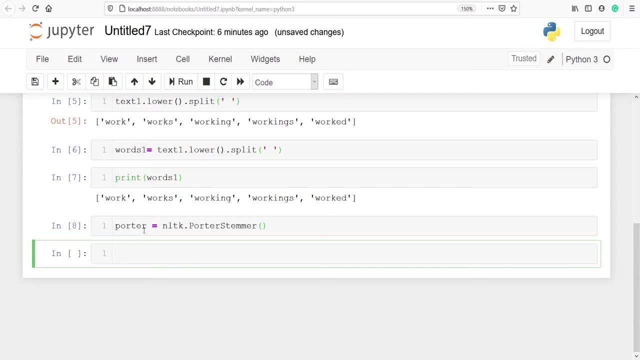 port stemmer class in the variable porter. This is an object of our port stemmer class And now I will run a for loop, I'll make a list, comprehension, Then I will say porterstem. So I have called this object porter. 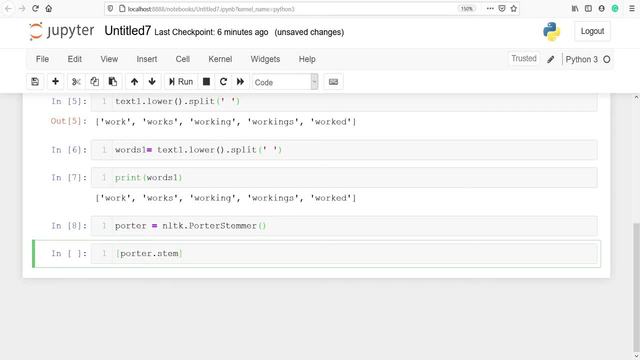 And from this object I am calling the method stem, w for w in words1.. So here I am writing a loop here. So I am saying that from the object porter, call the method stem And then for w in w words1, in this variable words1, apply it. 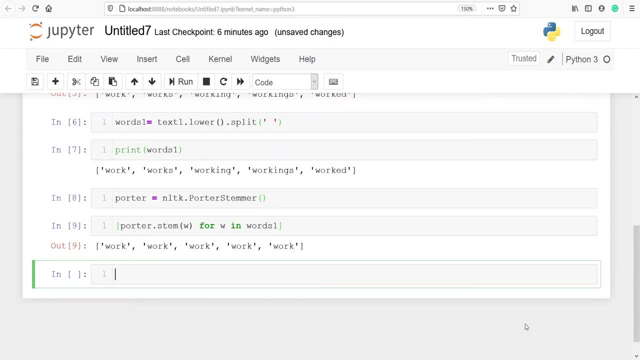 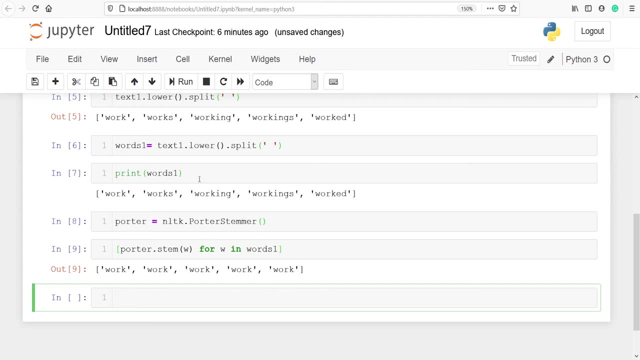 Let's execute our code In the output. you can see that now all the words are work, work, work, work and work. Earlier, we had work, works, working, workings and work. No matter whether it is work, working or anything, it will give you the stem of the word. That is the root of all this word. 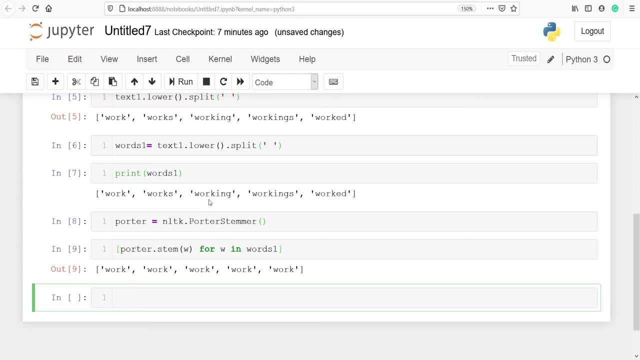 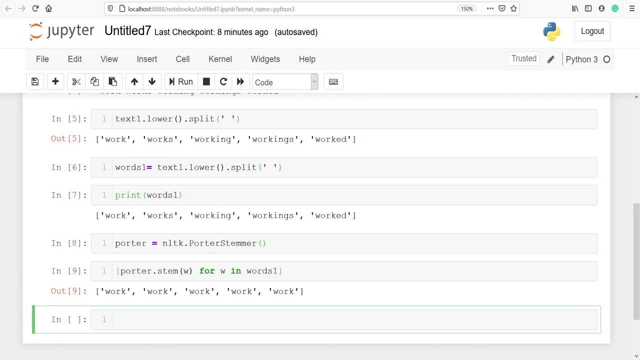 And if you see, the root of working is work. the root of working is also work. the root word of work is also work. This helps you to count the frequency of word work occurring how many times in a sentence. This is how stemming work. This video was about normalization and stemming in NLTK. 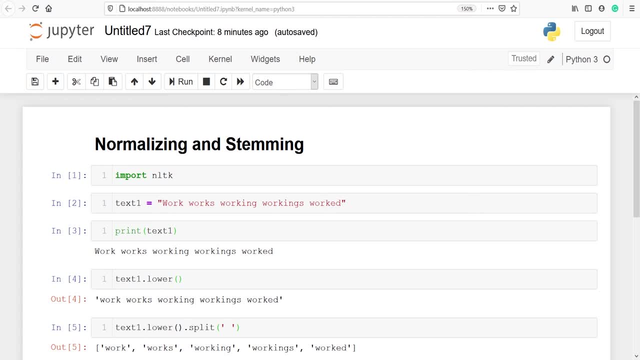 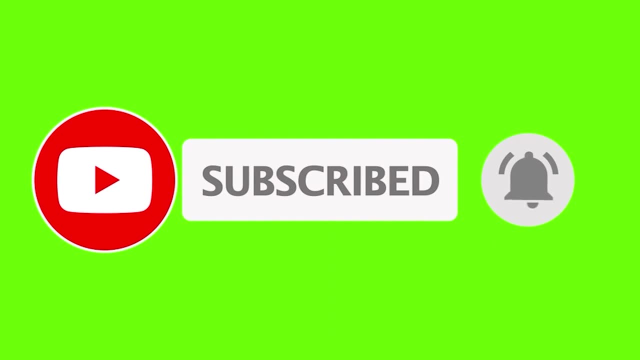 If you like my video, please subscribe to my channel. Thank you for watching.